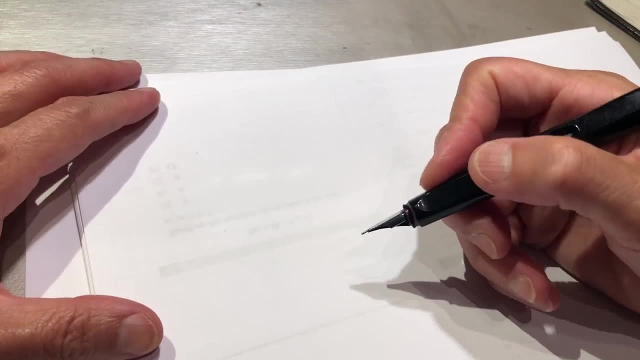 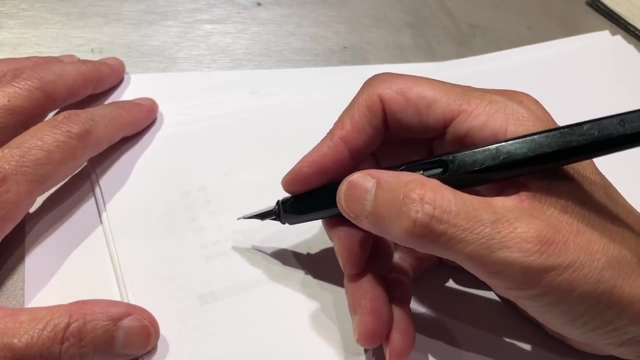 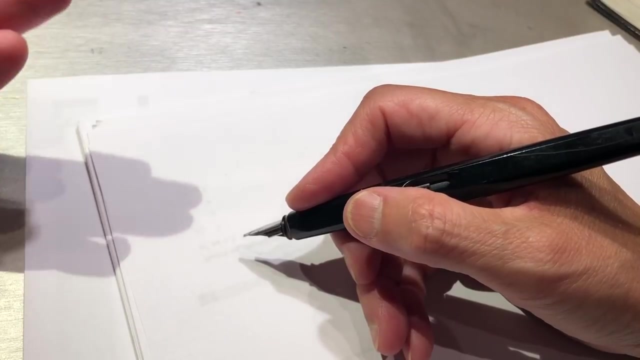 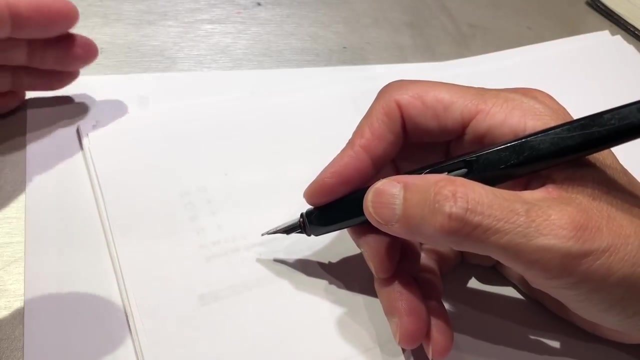 Okay, hello, dear friends. So today I was helping. working with one student on some simple arithmetic is a subtraction And, as I was doing, because we do it, we already do not need to think what is the method to do it. We just get the answer right Because our brain is already developed. 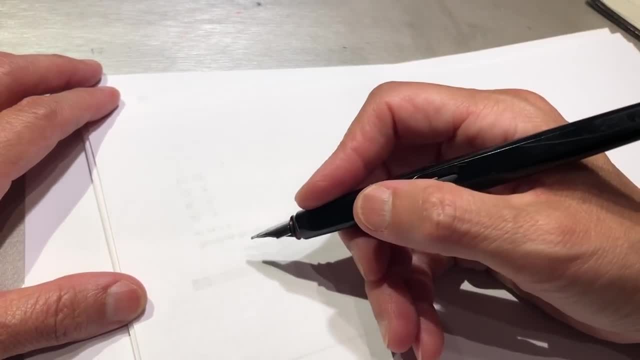 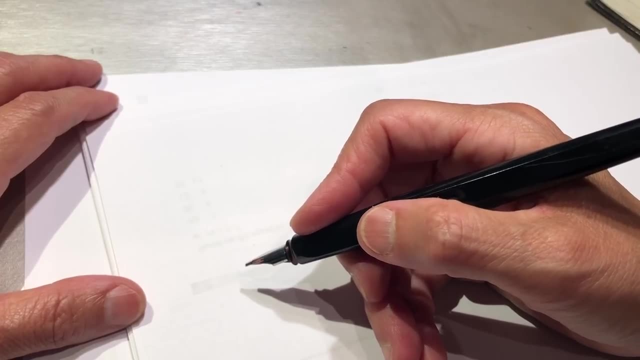 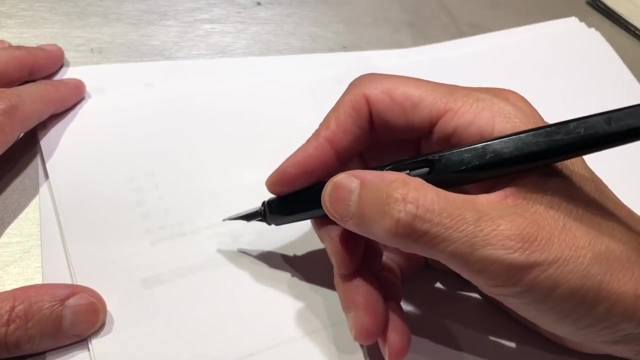 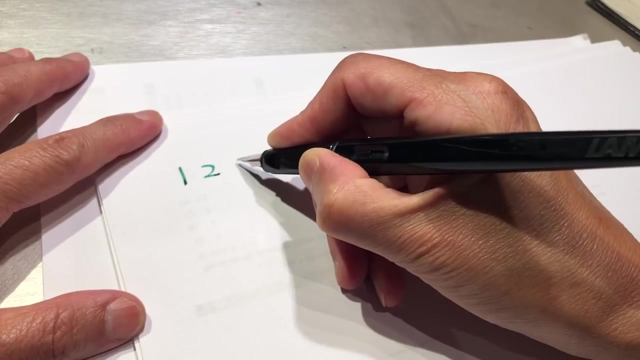 in such a level that we do not need to explain it. And then today I was trying to explain it and found it. It's actually quite interesting And it's kind of addicting. So I will just randomly choose some number: One, two, four, five, two Minus. 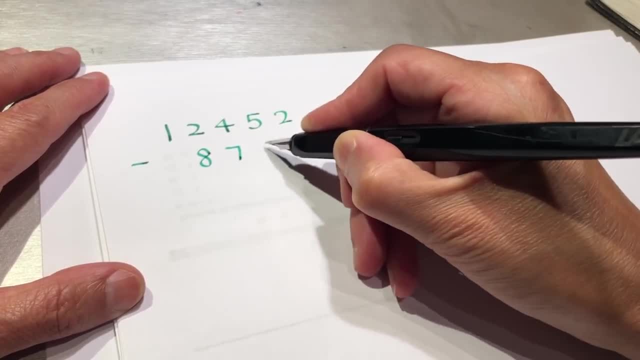 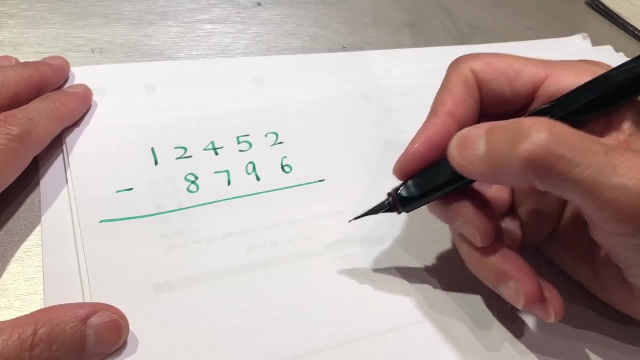 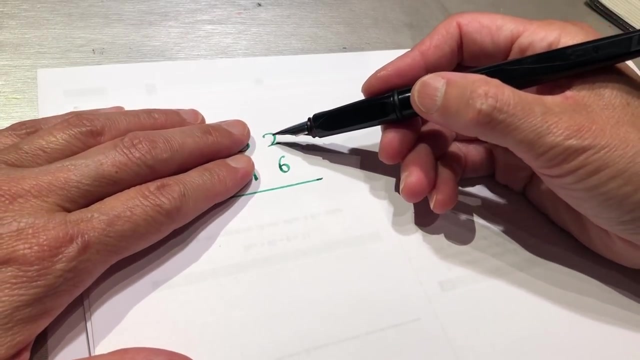 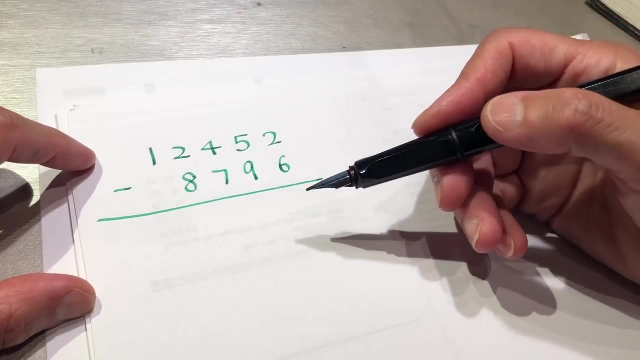 eight, seven, nine, six, because we want to use the method of borrow. How do we explain the borrow? Okay, how do we explain the borrow? So we do from the very right side, from the place value, the smallest place value, the ones, the tens, the hundreds, the thousands. 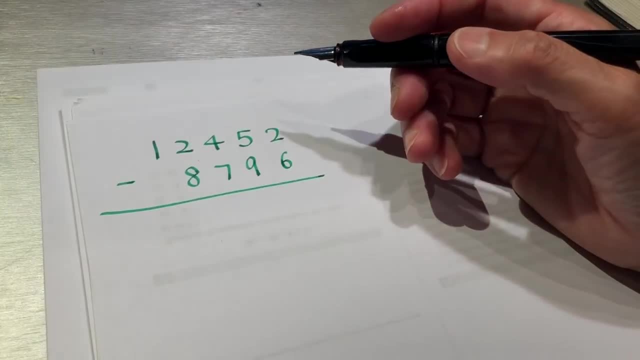 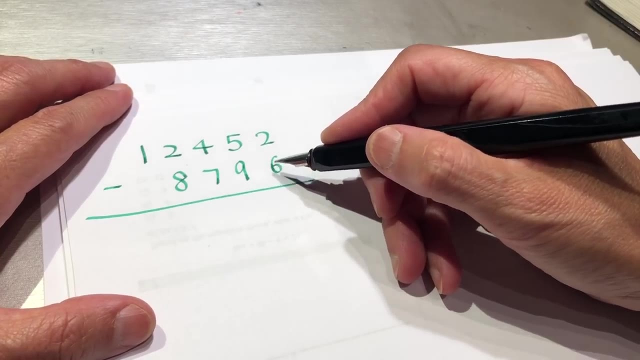 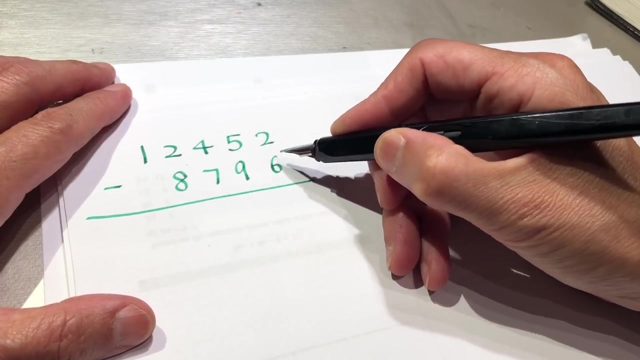 the tens of thousands, From smaller to large to big. Okay, two minus six. No, you cannot do it, because two is smaller. We are not yet learning about negative number. Two is smaller than six, So we need to go ahead. 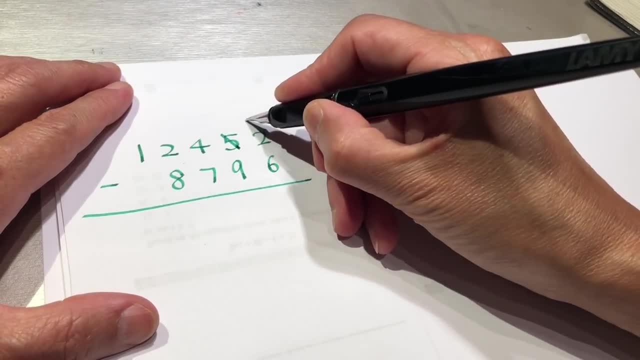 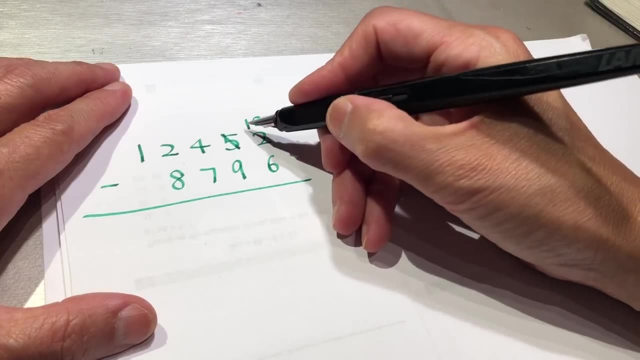 to borrow. And we borrow ten from the one before it, So it becomes twelve. We borrow ten from the one before it, So it becomes twelve. We borrow ten from the one before it, So it becomes twelve. We borrow ten from five, We borrow ten from five, Five from this. one is actually. 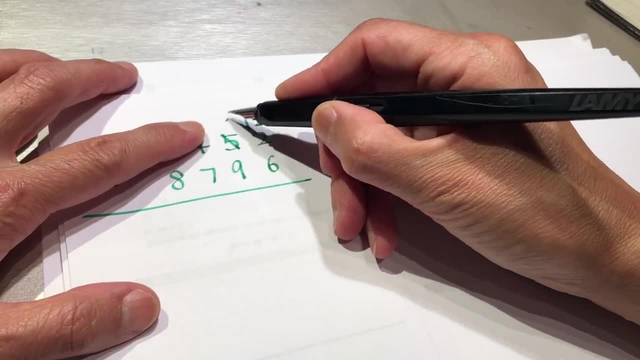 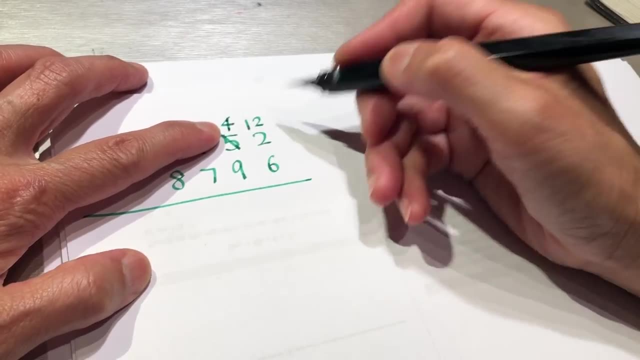 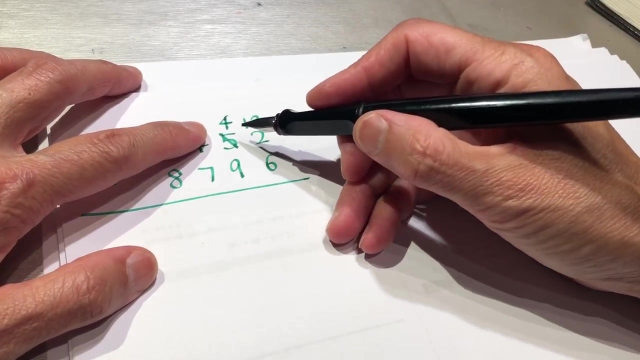 fifty right, We borrow ten from the tens value of five, Then the tens value of five have only four left because there was one goes to one level down. It's downgraded from alpha to beta. Okay, yeah, you know what I'm talking about. Twelve minus six. 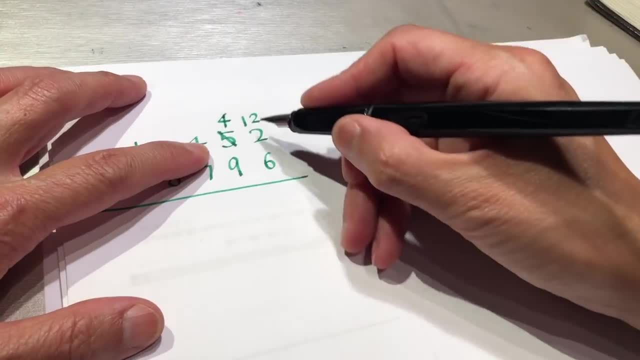 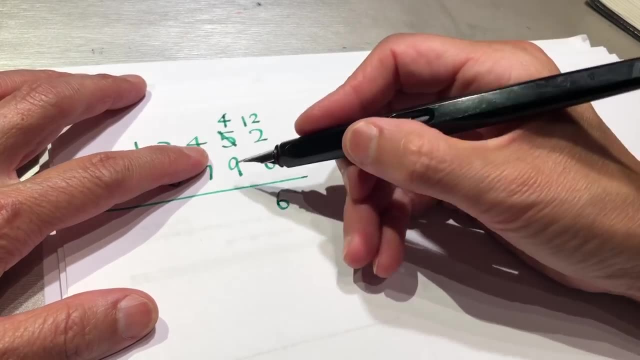 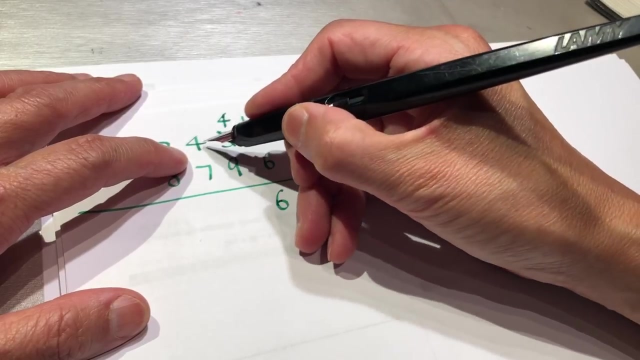 Can we do it? Yes, twelve is bigger than six, So twelve minus six is six. Now we need to do four minus nine. Four is smaller than nine, So we cannot do it. We need to go ahead to borrow And we go one step further. 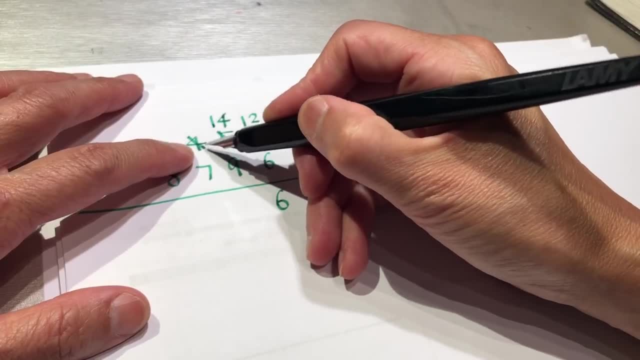 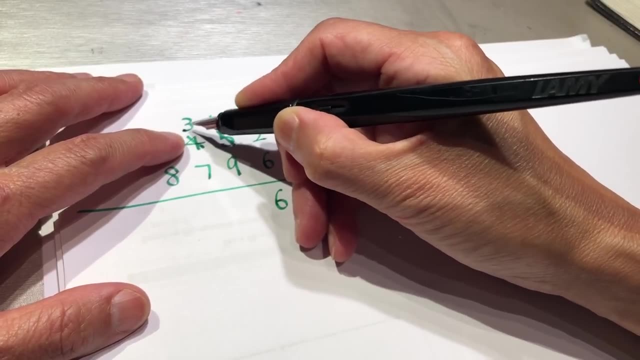 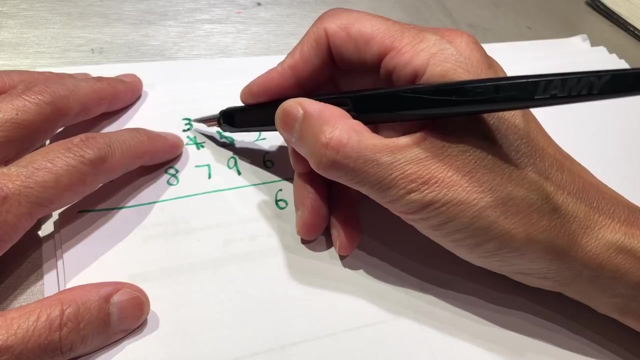 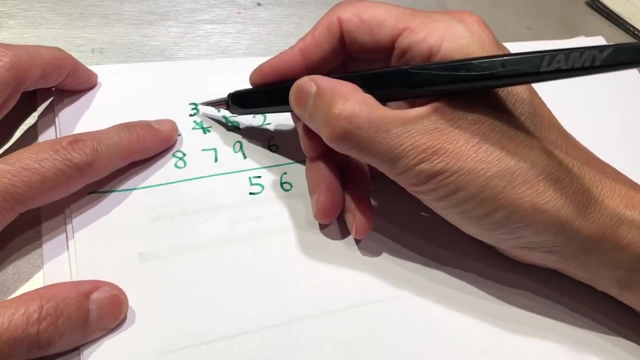 Here. from here borrow ten. And if we want to borrow ten here, we need to give ten, And the four is bigger than six. And the four gives one tenth away, becomes one three. Okay, So fourteen minus nine is five. We can do it. 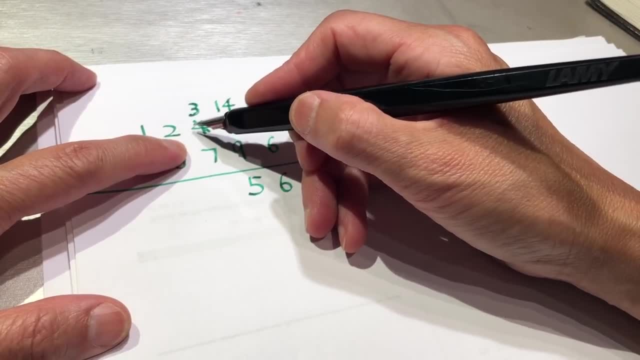 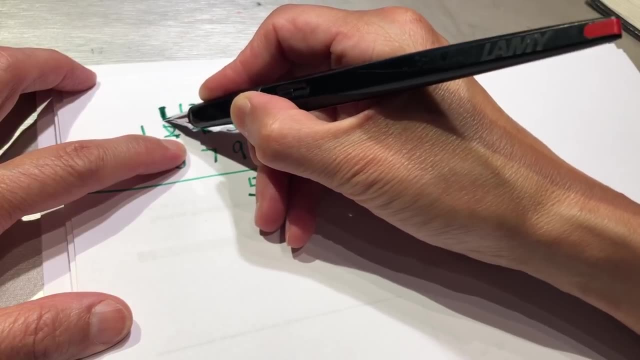 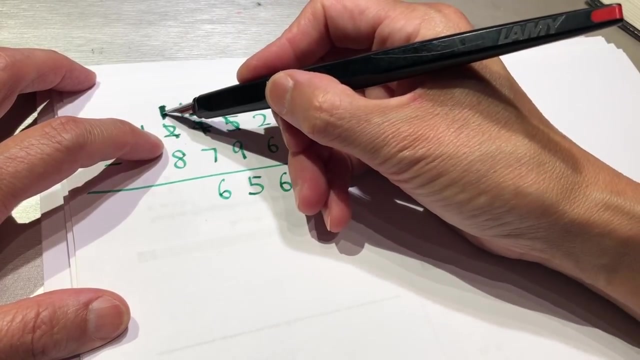 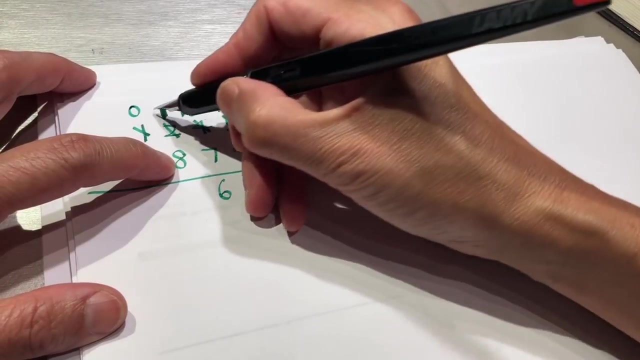 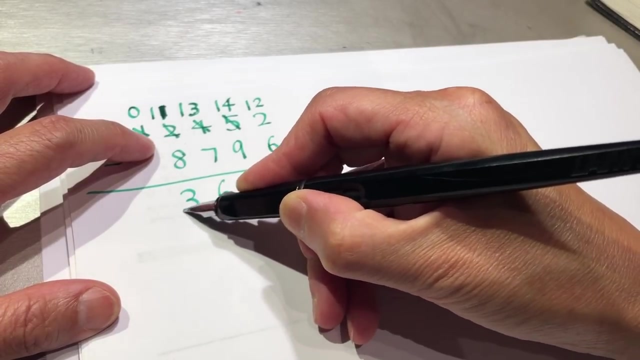 Now we need to. three minus seven. Three is too small. We need to borrow again. We borrow one, So two. borrow Two, give one. out becomes one. Thirteen minus seven is six. One minus eight is still too small. We need to borrow. Borrow one. This one becomes zero And here becomes eleven. Eleven minus eight becomes three. 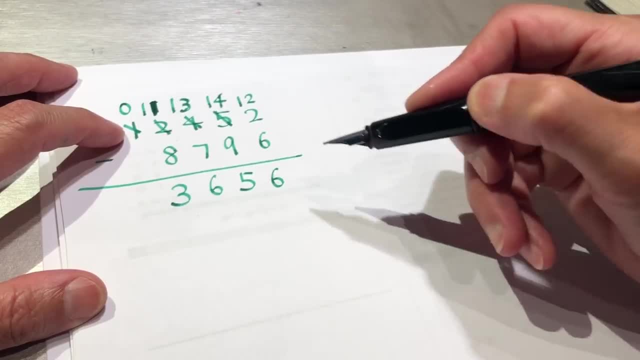 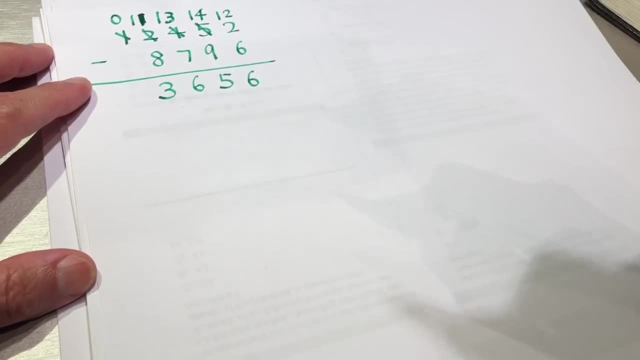 So the answer is three, six, five, six. So this is the method of doing it. Now we will do another method. Okay, this question, we will do another method. This question, we will do another method. 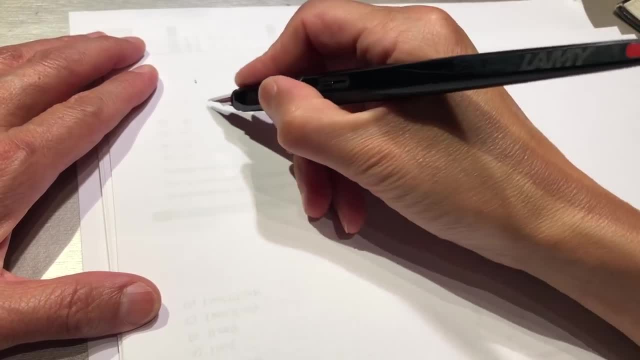 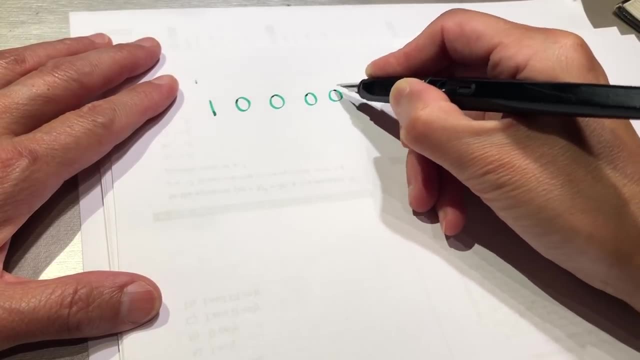 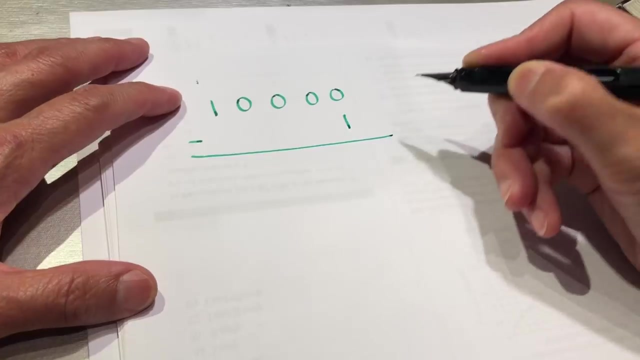 Okay, this question, we will do another method. This question, we will do another method. We will do something that we all know, but how we explain it? Ten thousand. So this is Ge Shi by Jie Wan. Ten thousand minus one. We know it's 9,999, right, But how do we get it? 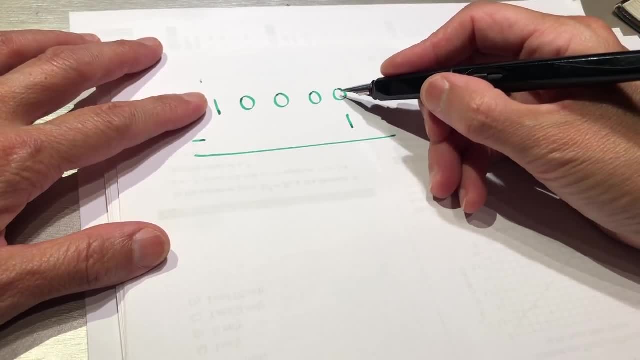 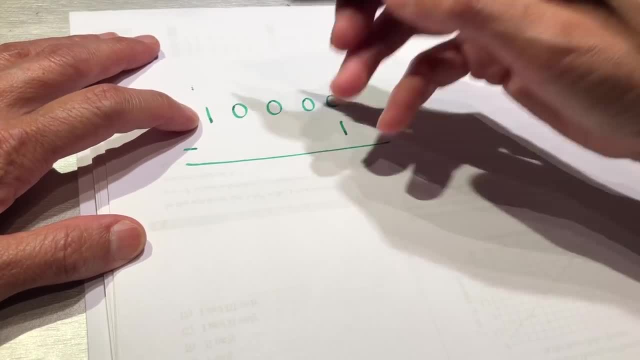 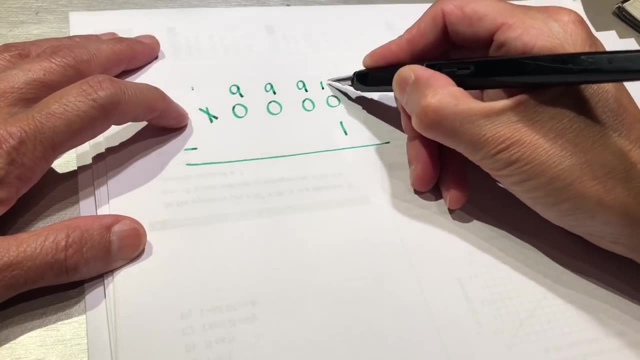 So we have ten thousand, and we will do from the very left, step by step. So we have ten thousand and we will do from the very left, step be step, and then will do from the very right, step by step. 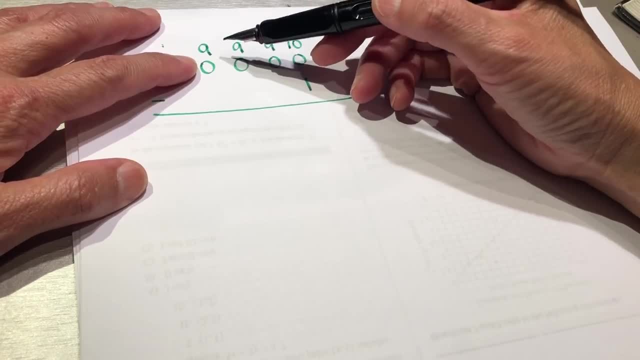 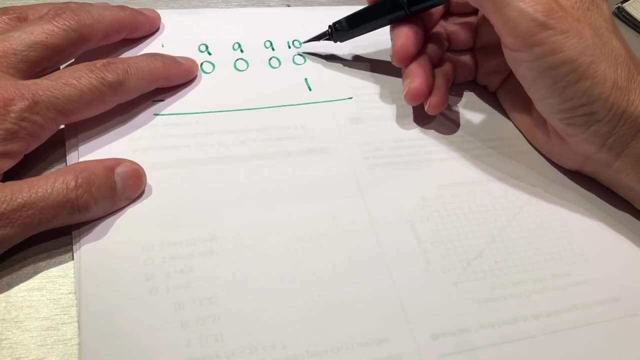 So there is essence in the small one. So there is essence in the small one. If we see the place value of the writing means So 9,990.. and valid for 10.. Each of these is one place value. 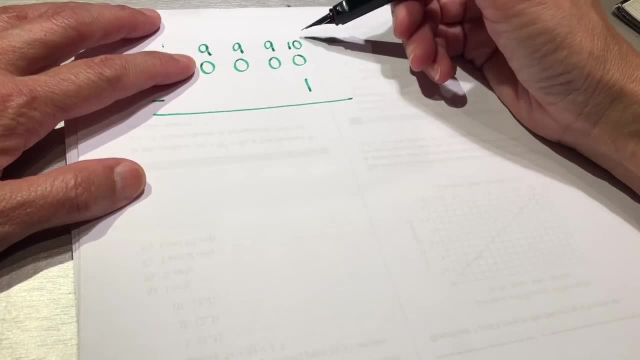 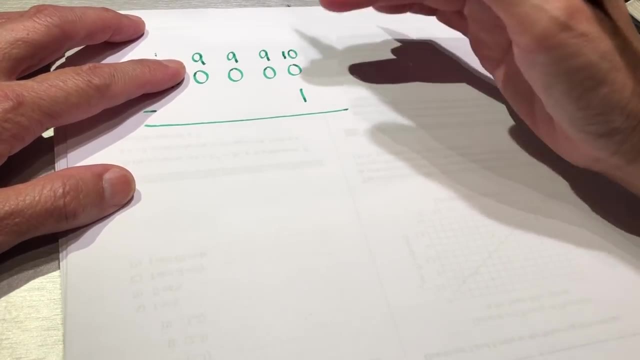 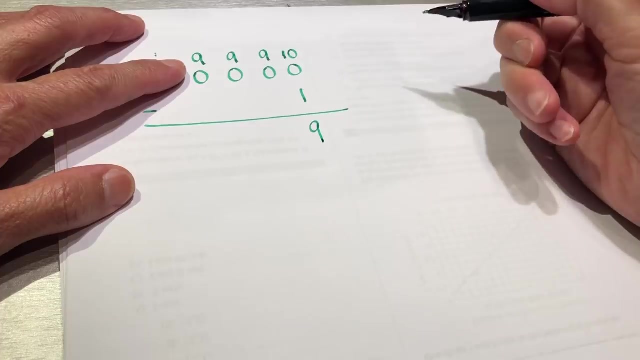 9,990 plus 10, and together it makes 10,000,. right, And this way we can start to do the subtraction. 10 minus 1 is 9. 9,, nothing below it, it just copy it. 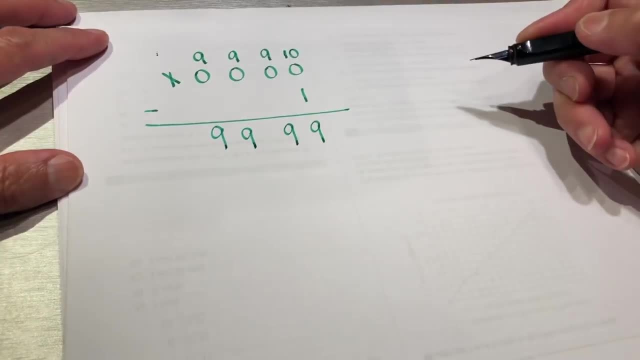 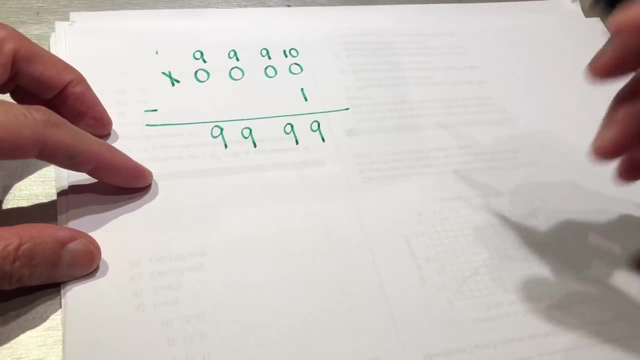 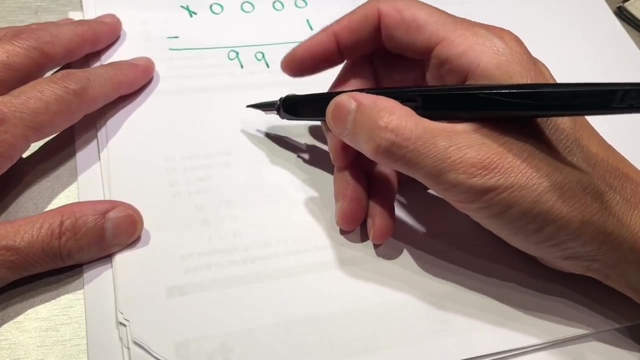 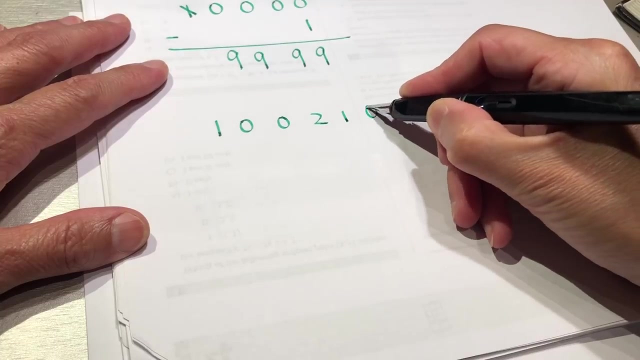 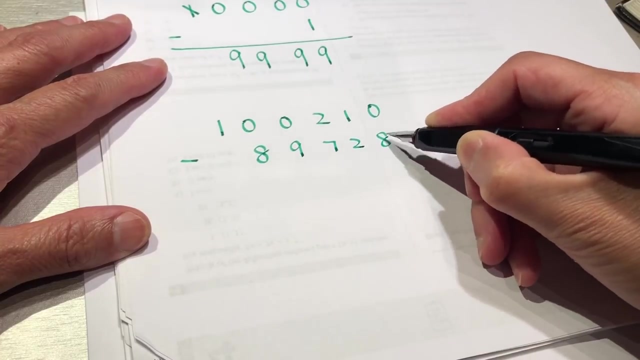 9, 9, 9.. Do I make sense? So we just need to keep on borrow, borrow, borrow until we get that money we need? Okay, this one. we will do the number a little bit more interesting: 1, 0, 0, 2, 1, 0 minus 8, 9, 7, 2, 8.. 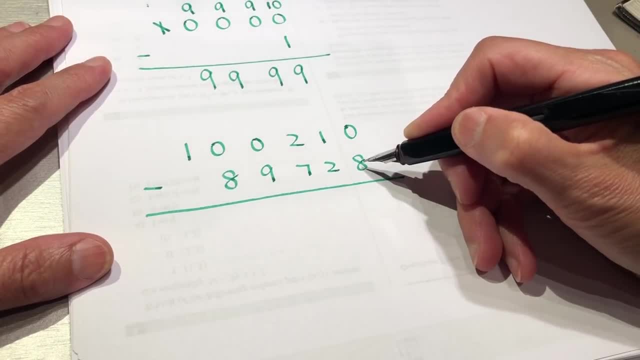 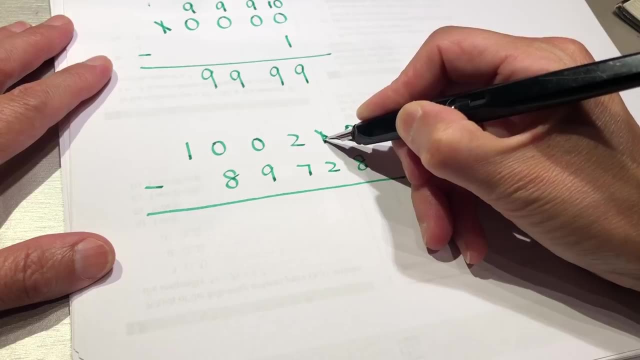 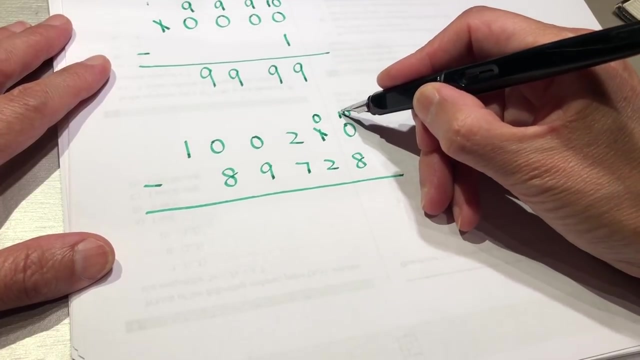 0 minus 8, uh-oh, not enough, so we need to go ahead to borrow. We borrow from 1,. 1 becomes 0, and this 0 in 1 becomes 10, right, 10 minus 8 is 2.. 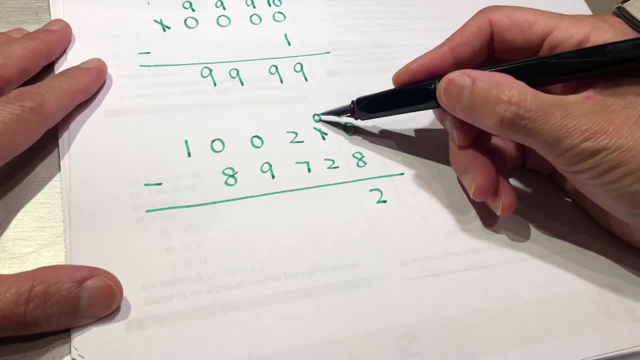 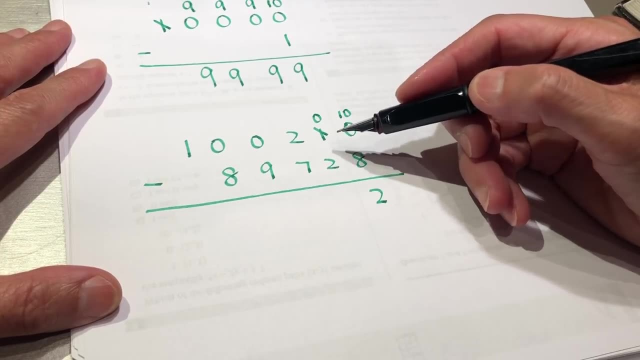 Good, we can do it. Okay now. the next one is 0 minus 2.. Uh-oh, 0 is 2.. 1 is smaller than 2, so we cannot do it. We still need to borrow. We borrow 1, becomes 1, 10.. 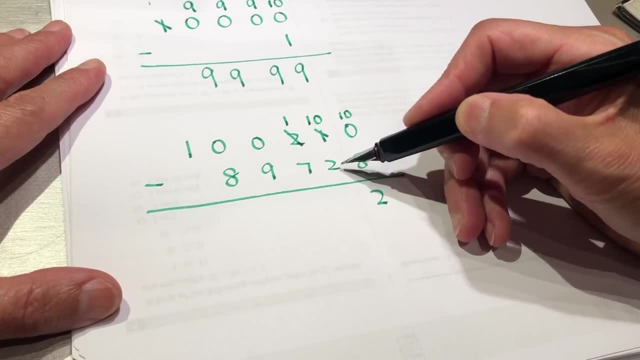 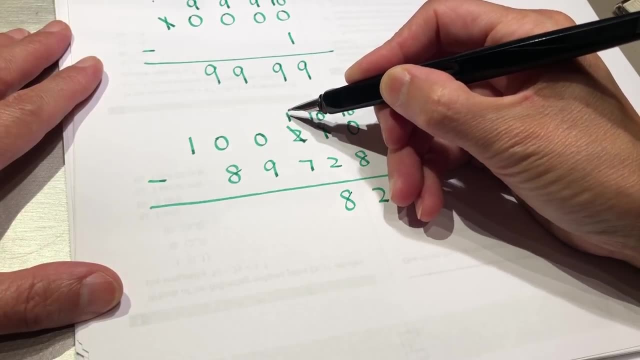 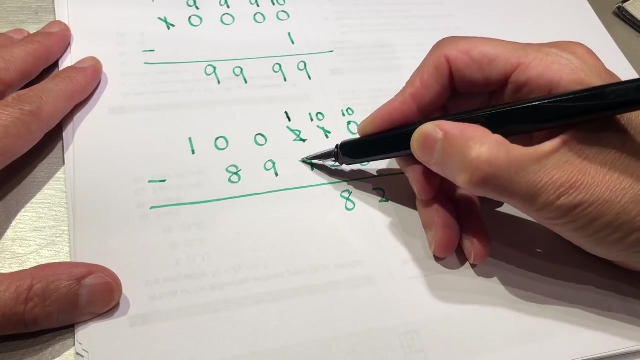 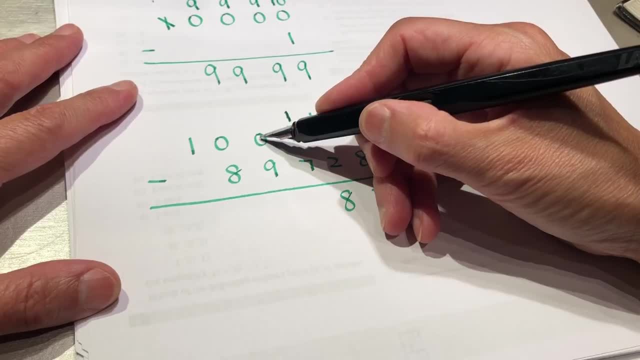 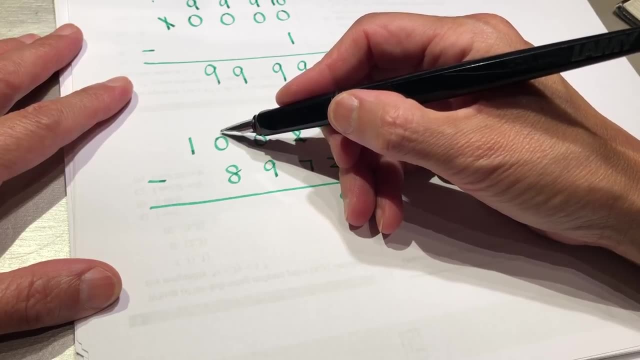 1. 1., 1., 1., 1. 1. 1.. And it does not have. there is nothing for us. We need to go to the next door. There is still nothing for us. We go to even next door. 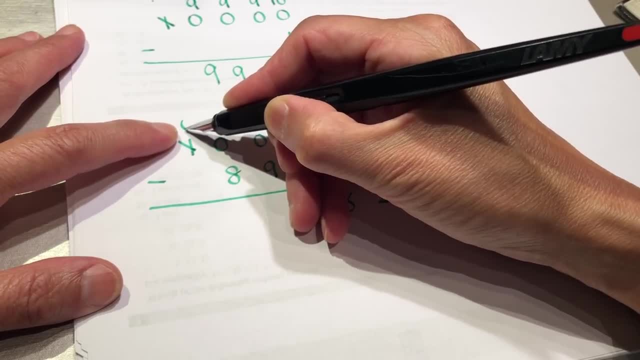 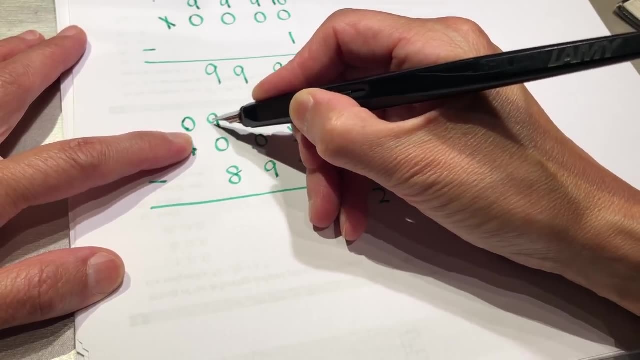 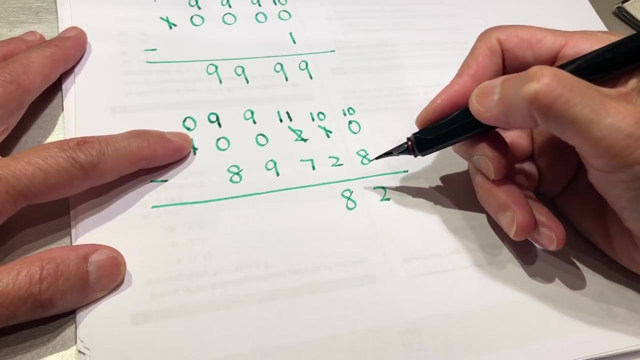 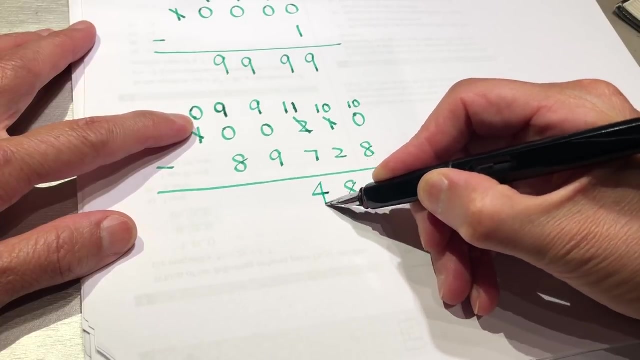 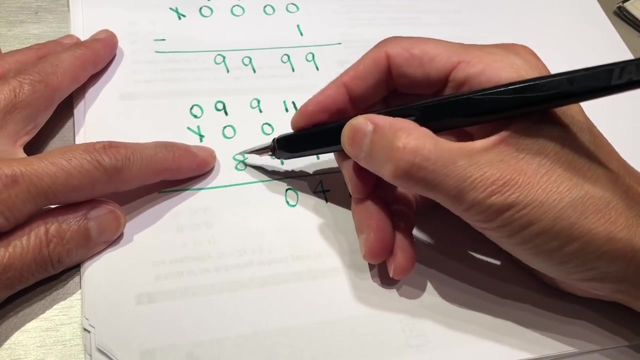 Oh, we can borrow And it lands us 1, but this 1 becomes 9,, 9 and 11.. 1.. okay, so 11 minus 7 is 4, 9 minus 9 is 0, 9 minus 8 is 1, so the result is 1, 0, 4, 8, 2. 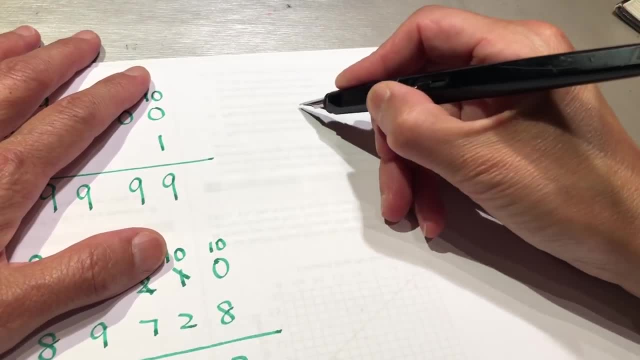 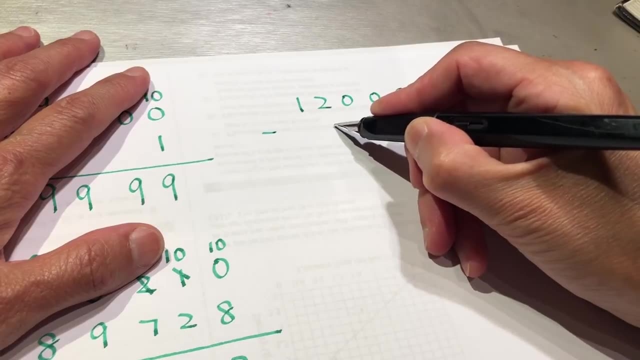 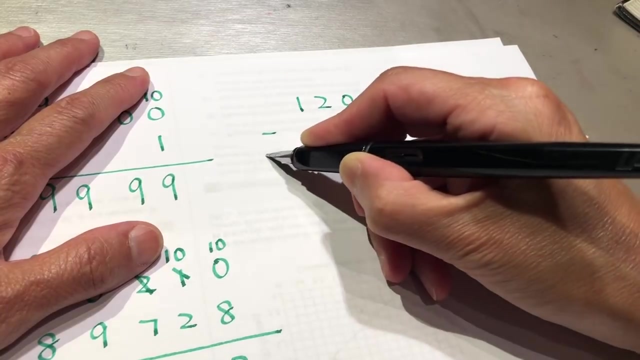 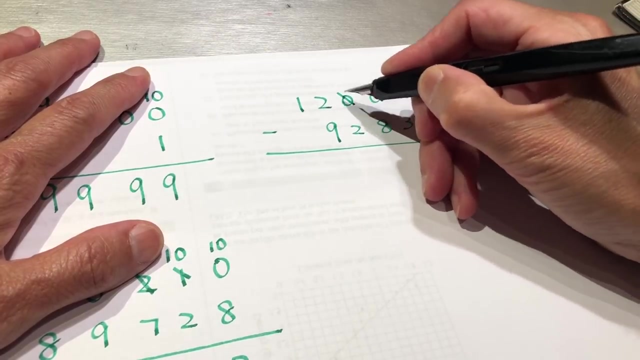 let's do another. uh, 0, 1, 1, 2, 0, 0, 0, 5 minus 9, 2, 8, 7, 8, 8, 5 minus 8. no, go ahead, borrow 1, 9, 9, 9, 15. 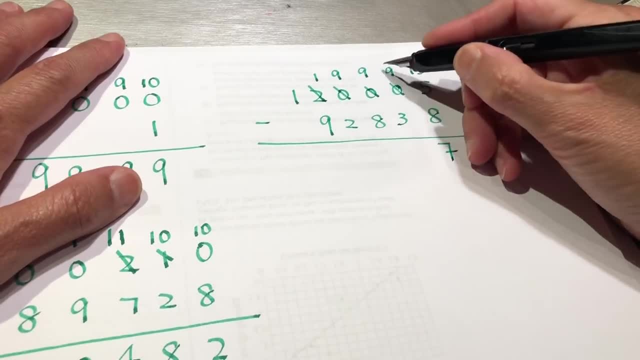 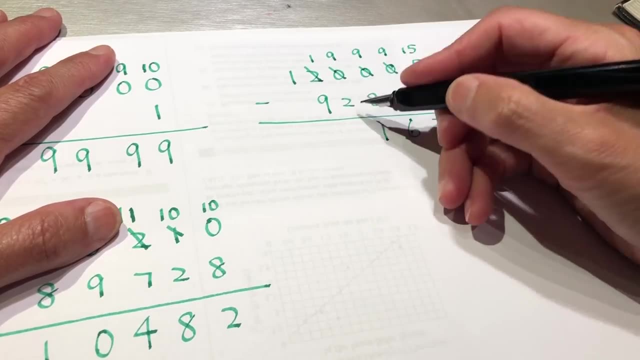 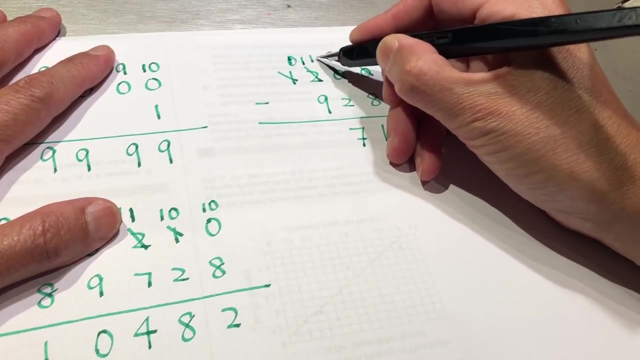 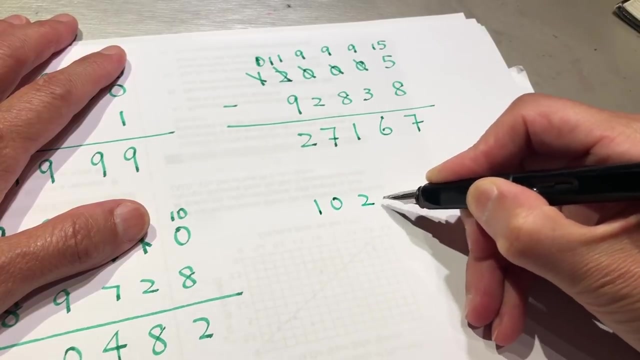 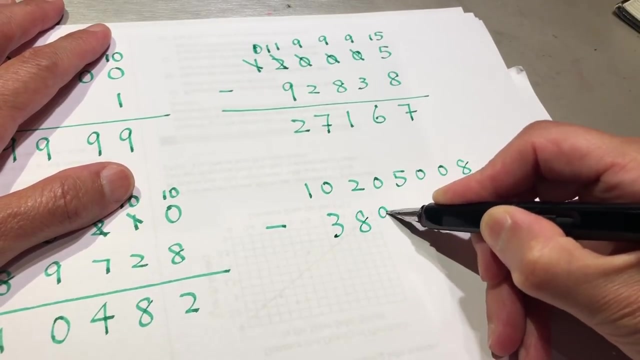 15. 15 minus 1 is 7, 9 minus 6 is 9 minus 3 is 6. 9 minus 8 is 1, 9, 2, 7, 1 still oh, 11 minus 9 is 2, 2. 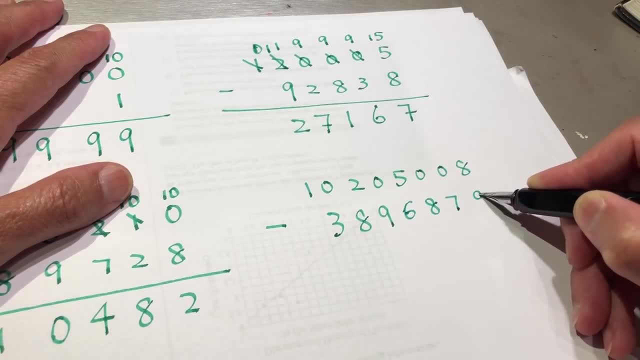 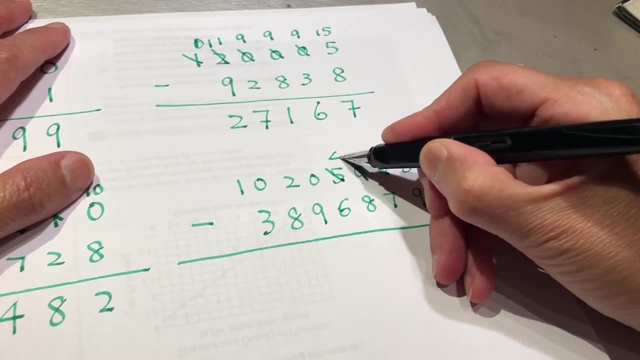 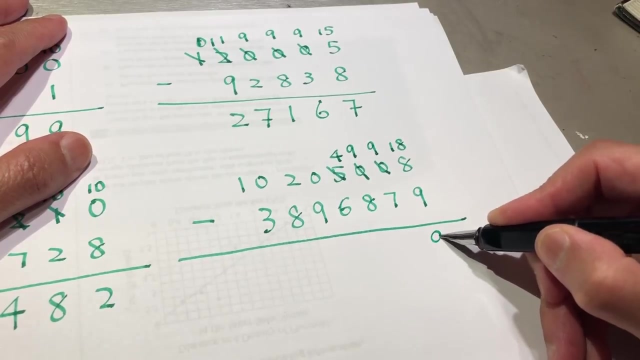 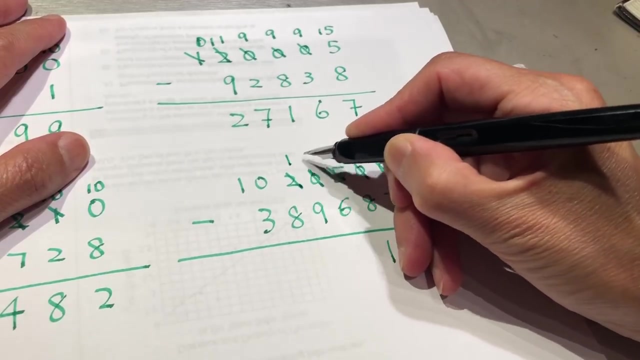 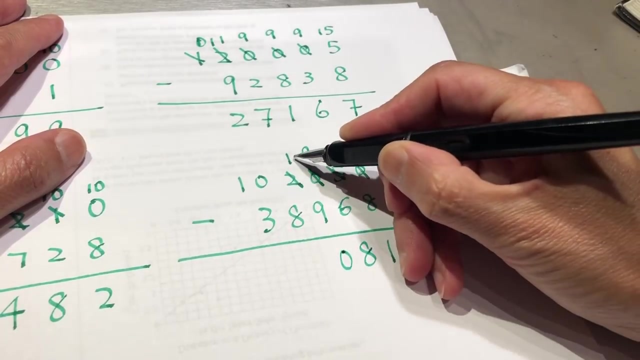 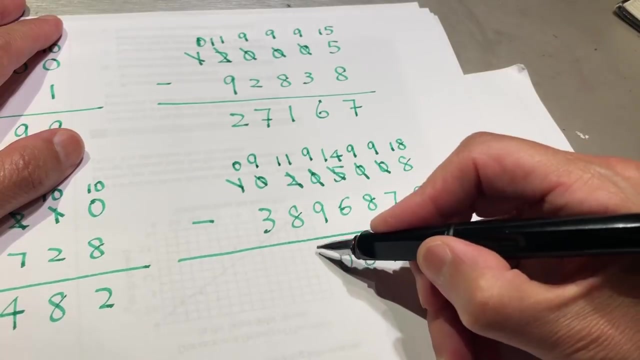 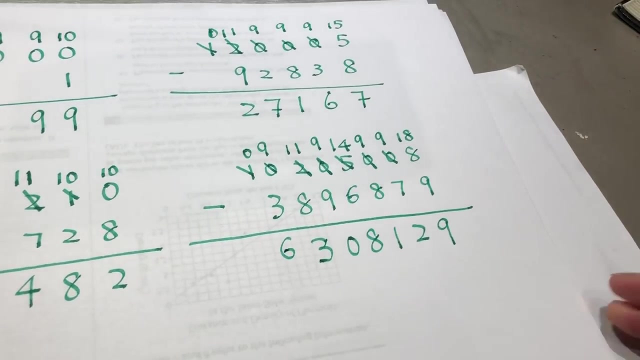 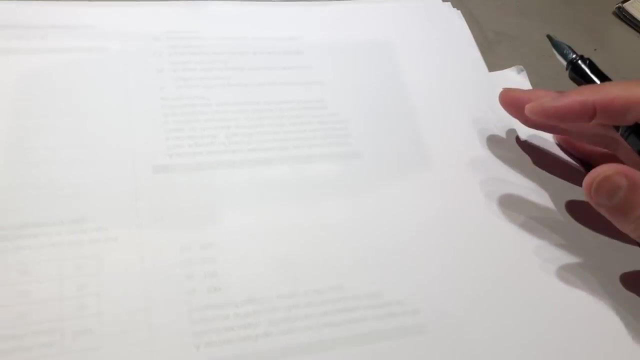 2, 8. no 89: 2, 1 o o not enough. 4, 14,, 8, 0,. hmm, not enough: 11, 3. Okay, so we can just do like this. Let me continue to do something without even talking. 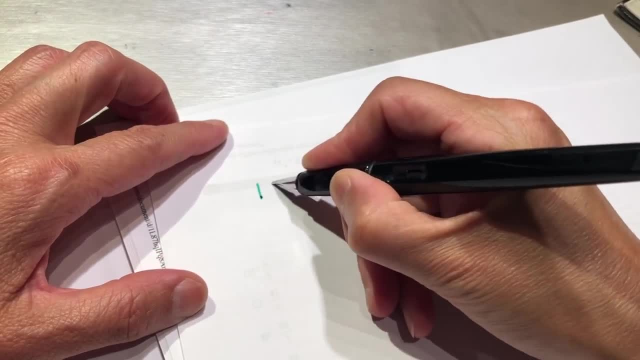 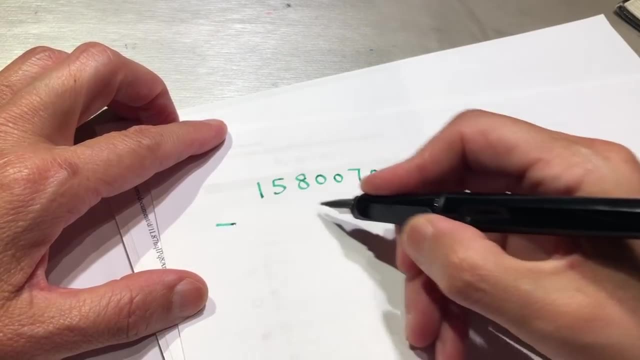 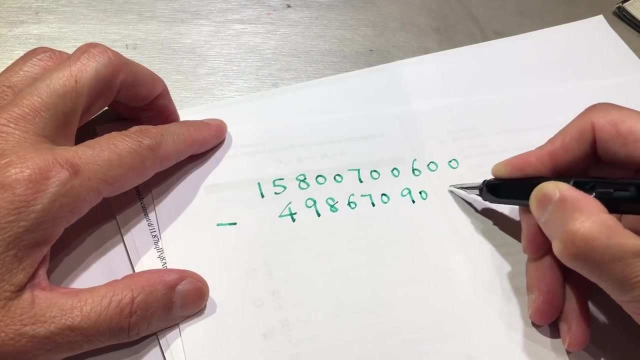 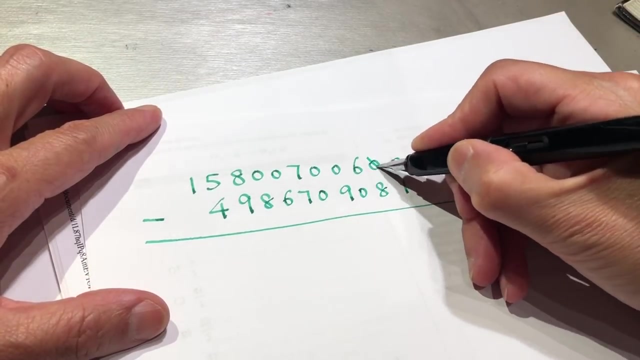 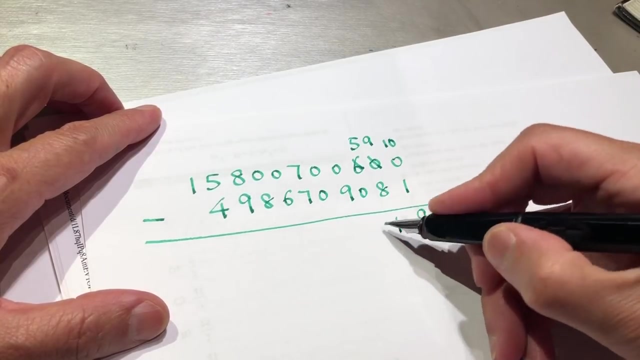 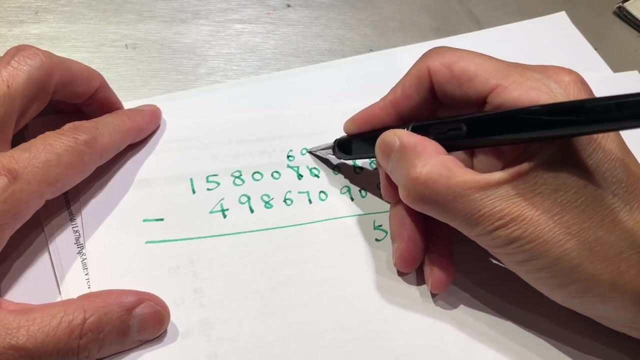 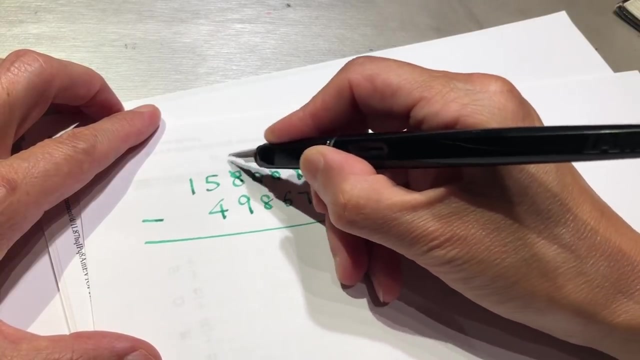 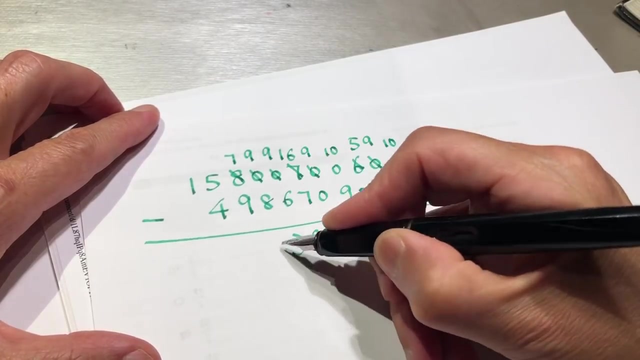 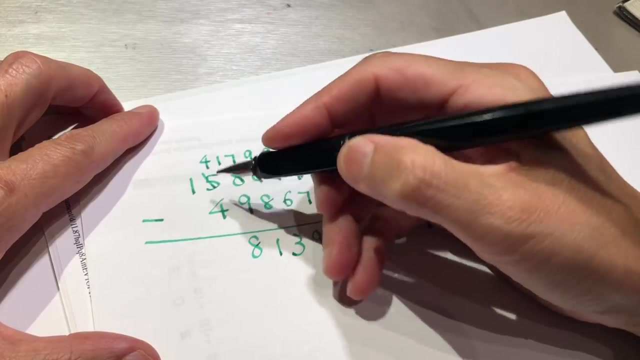 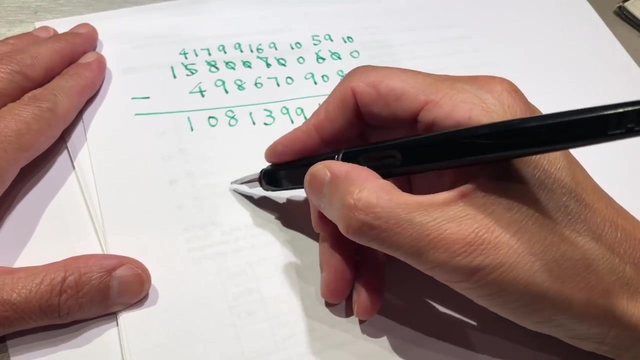 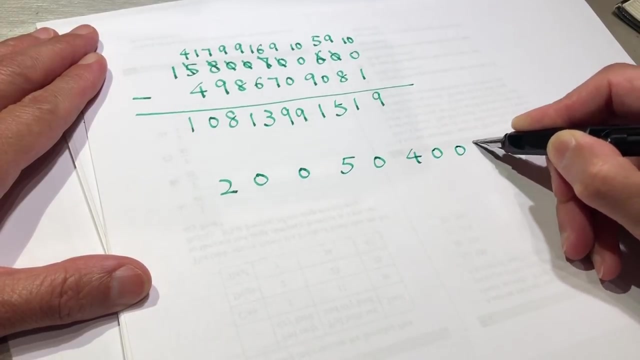 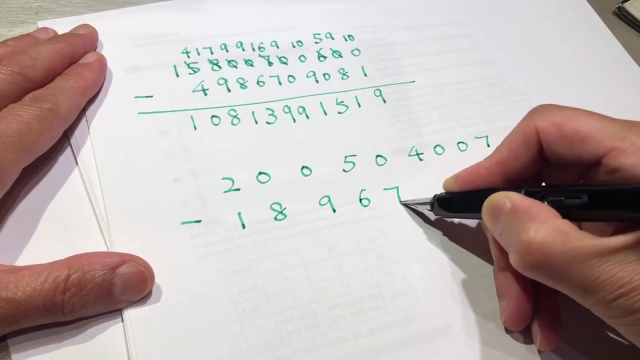 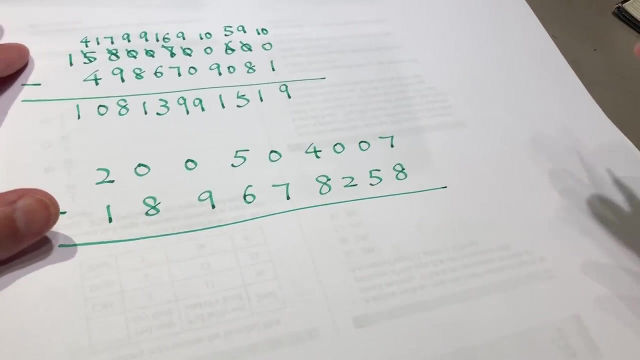 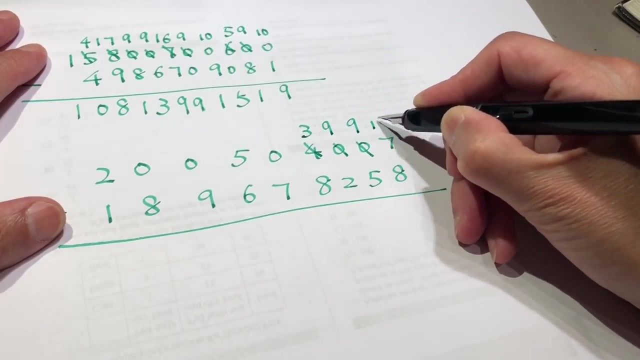 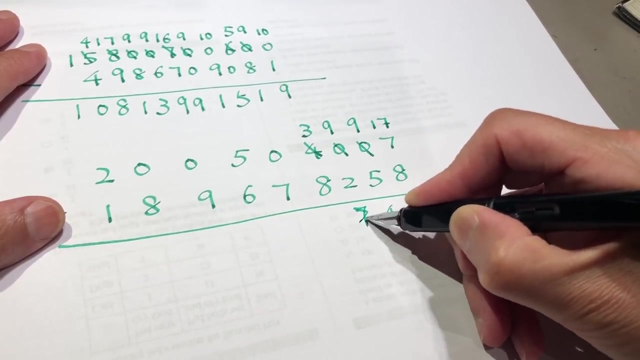 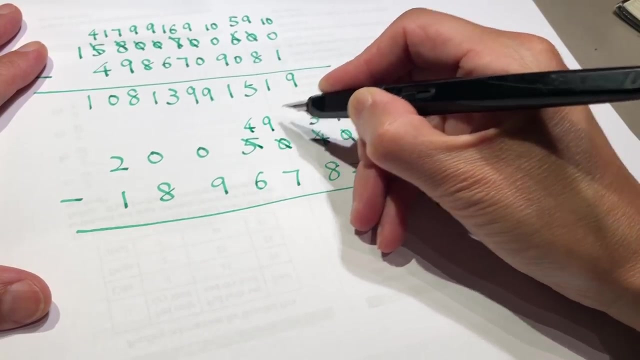 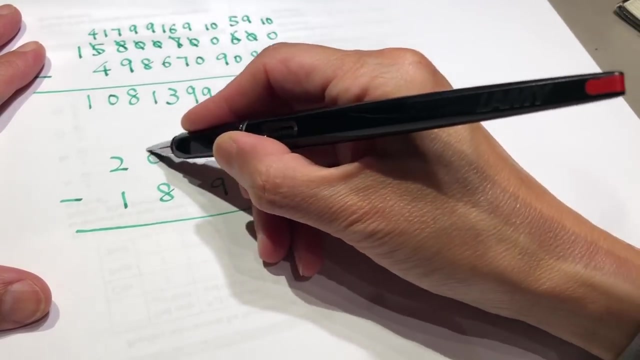 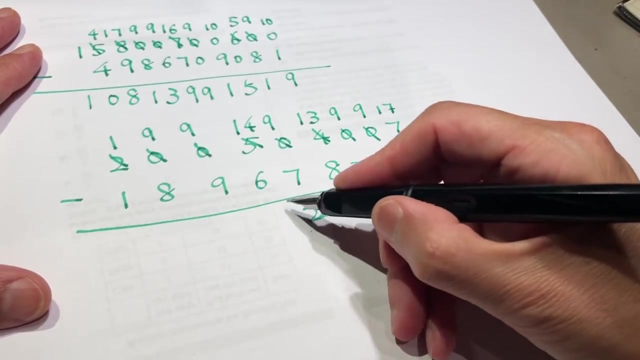 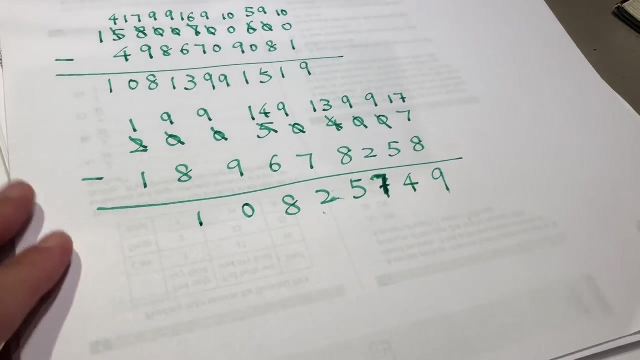 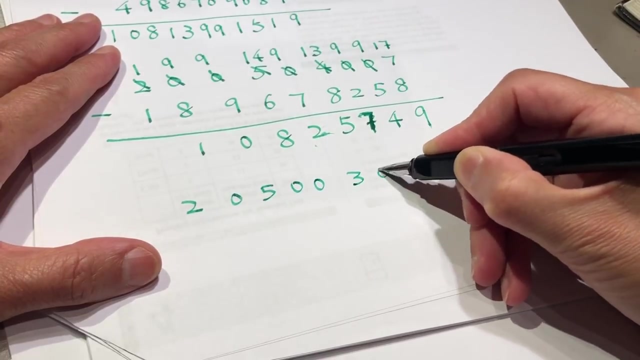 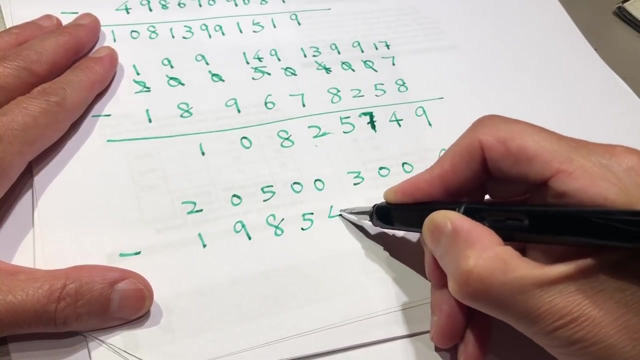 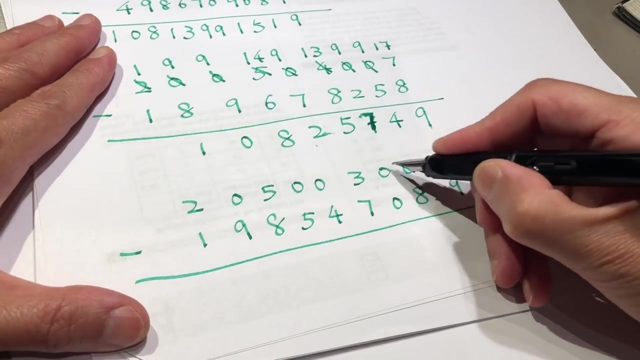 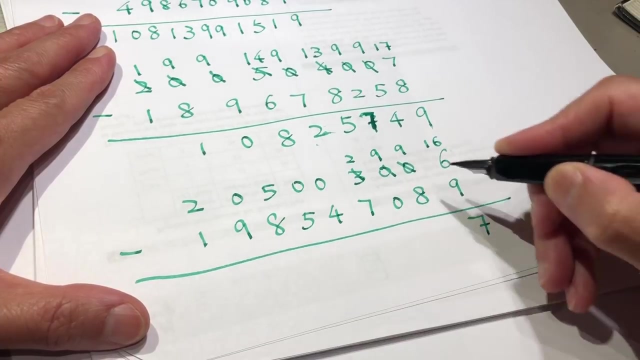 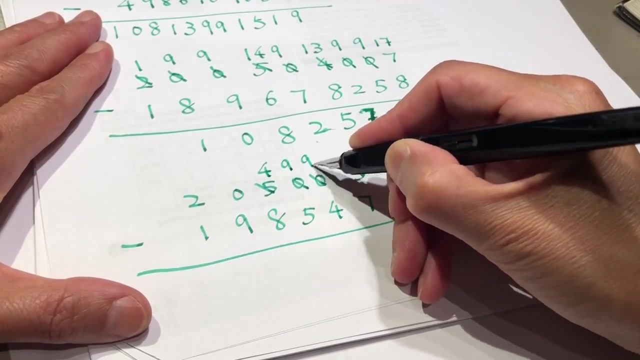 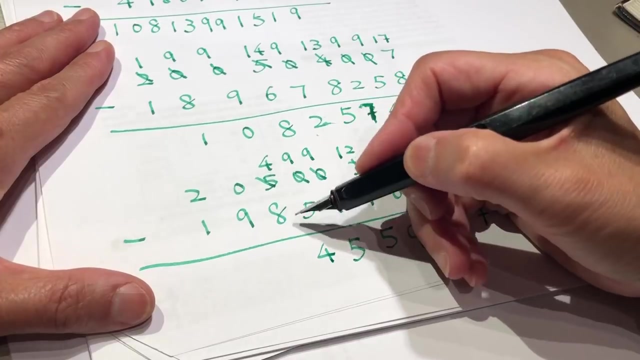 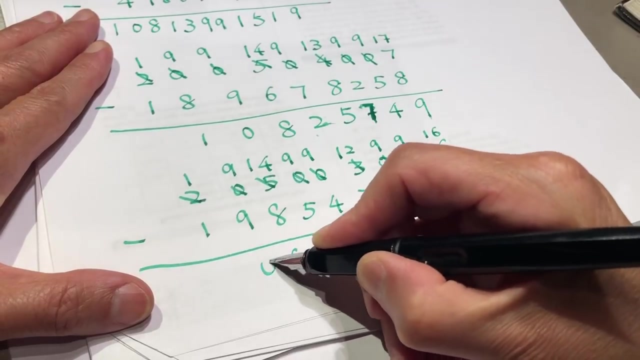 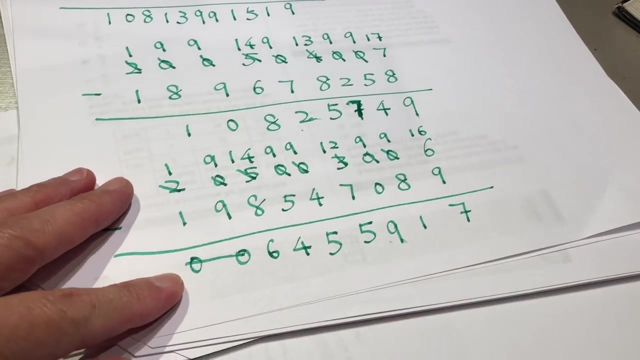 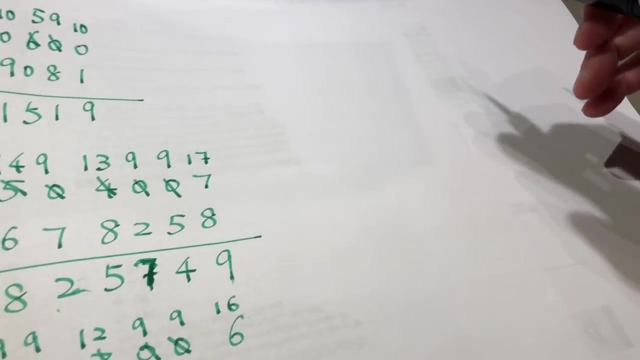